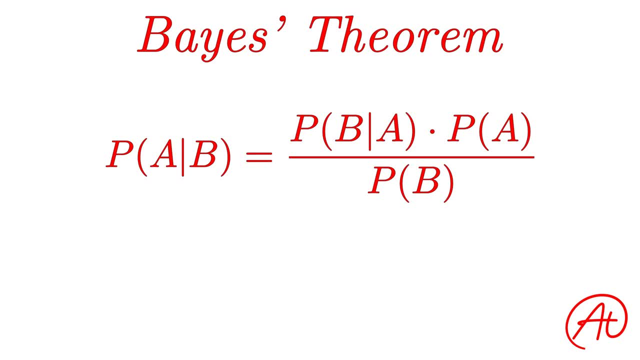 of B. Okay, I know that was a mouthful and I know this can look a little confusing, so let's first discuss when you would actually use this and where it comes from. So, first off, this formula is being used to calculate the probability of A given B In other. 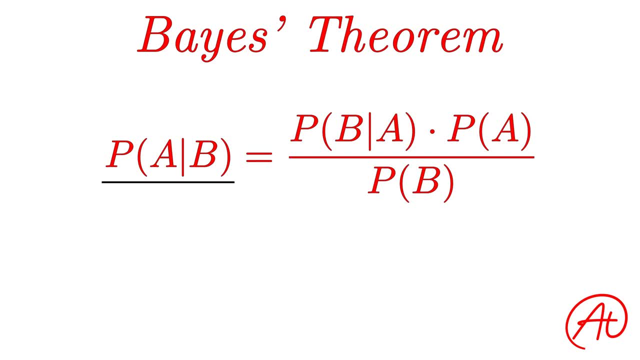 words. this is figuring out what the probability of a certain event occurring is, given that we already know that another event occurred. If you already watched our video on probability formulas, then you may recall that the general formula for a conditional probability like this is the. 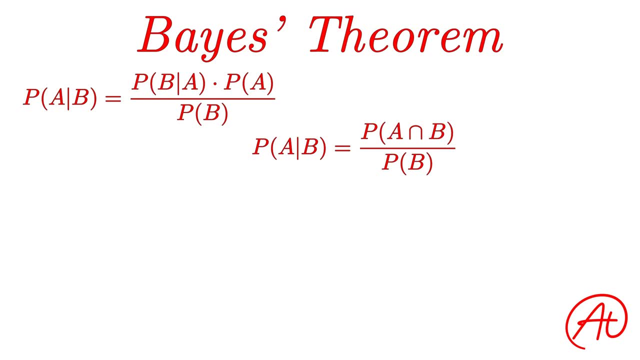 probability of A and B occurring divided by the probability of B. With this formula, we are just one step away from getting Bayes' Theorem. The one thing we need to replace in this formula is the probability of A and B right up here And 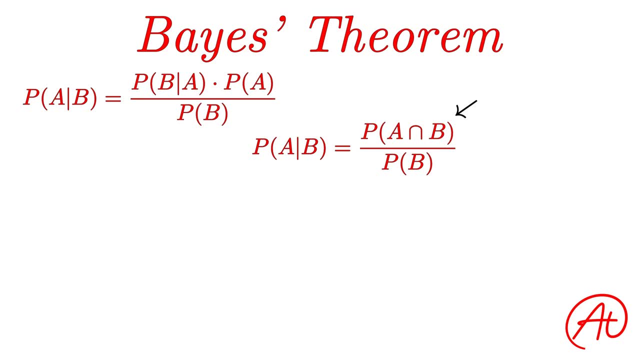 we can replace this value if we look at the same conditional formula, but the other way around. To see what I mean, let's swap around B and A. to get the probability of B given A is the probability of B and A divided by the probability of A. Now I know I may have gone a little fast through that. 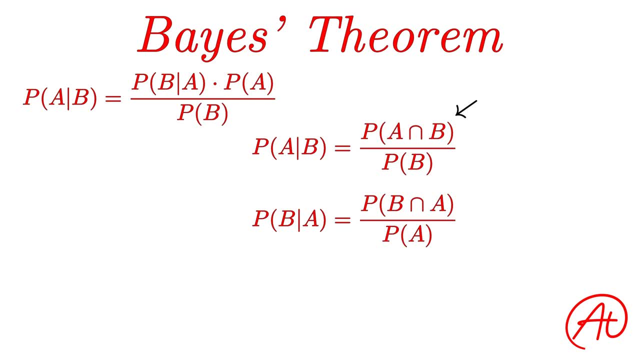 but all we did was take the normal conditional formula of the probability of A given B and just swap all of the B's for A's and A's for B's. Keep in mind we're looking to replace the probability of A and B here. 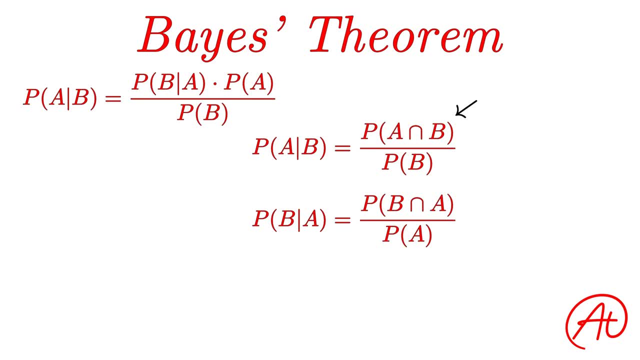 Well, in this equation below, we can see something that looks pretty similar: the probability of B and A. If you recall from our previous video, the probability of A and B is called the intersection of A and B, And if you look at the Venn diagram describing these two events, 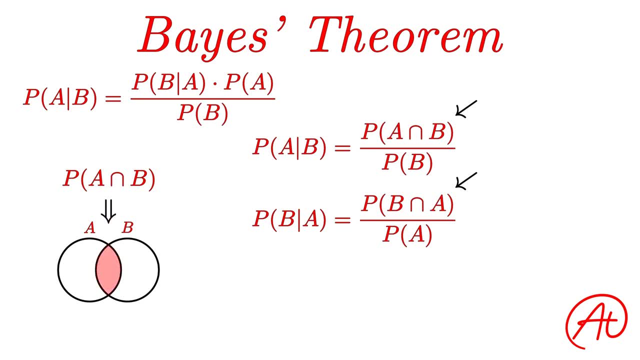 the intersection of A and B is right here, where the two events circles intersect. One thing to note here is that it doesn't matter whether it's the probability of A and B or B and A. It still just refers to the same thing: the overlapping portion of the two events. 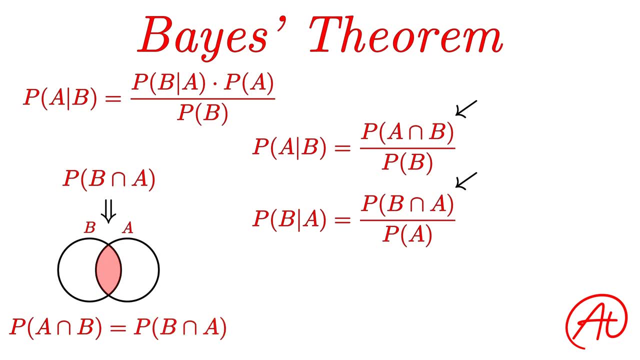 So the probability of A and B is equal to the probability of B and A. With that fact, we can now replace this probability of B and A with the probability of A and B, so it looks closer to the equation we have above. 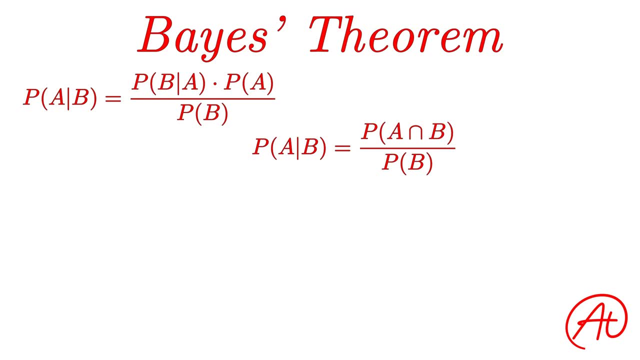 probability of A and B occurring divided by the probability of B. With this formula, we are just one step away from getting Bayes' Theorem. The one thing we need to replace in this formula is the probability of A and B right up here And 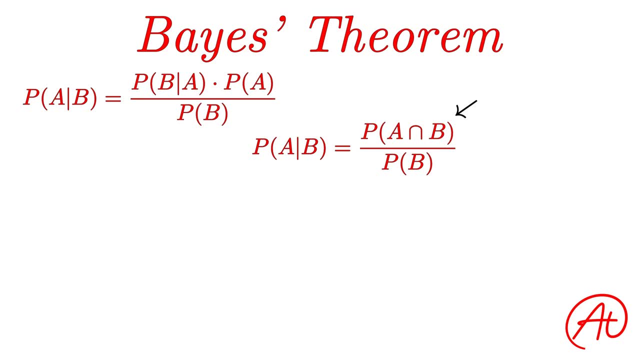 we can replace this value if we look at the same conditional formula, but the other way around. To see what I mean, let's swap around B and A. to get the probability of B given A is the probability of B and A divided by the probability of A. Now I know I may have gone a little fast through that. 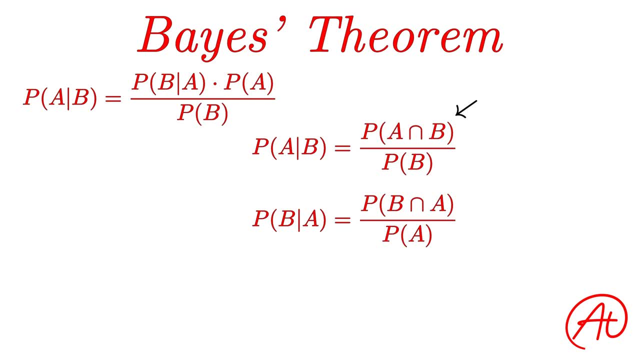 but all we did was take the normal conditional formula of the probability of A given B and just swap all of the B's for A's and A's for B's. Keep in mind we're looking to replace the probability of A and B here. 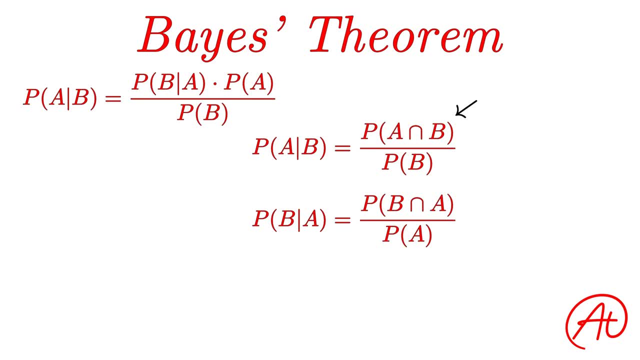 Well, in this equation below, we can see something that looks pretty similar: the probability of B and A. If you recall from our previous video, the probability of A and B is called the intersection of A and B, And if you look at the Venn diagram describing these two events, 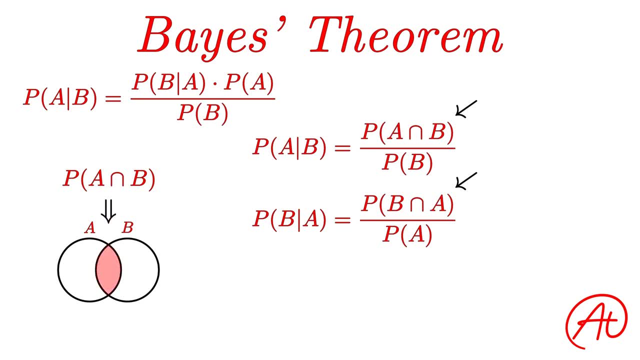 the intersection of A and B is right here, where the two events circles intersect. One thing to note here is that it doesn't matter whether it's the probability of A and B or B and A. It still just refers to the same thing: the overlapping portion of the two events. 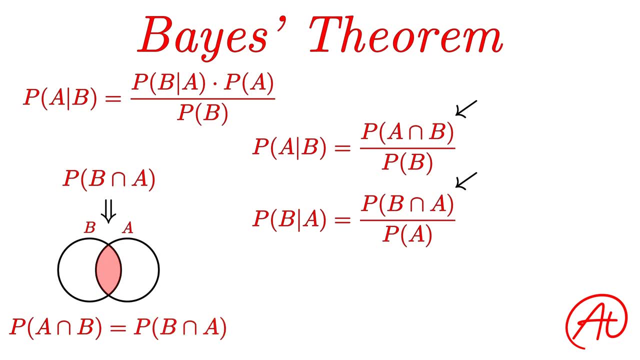 So the probability of A and B is equal to the probability of B and A. With that fact, we can now replace this probability of B and A with the probability of A and B, so it looks closer to the equation we have above. 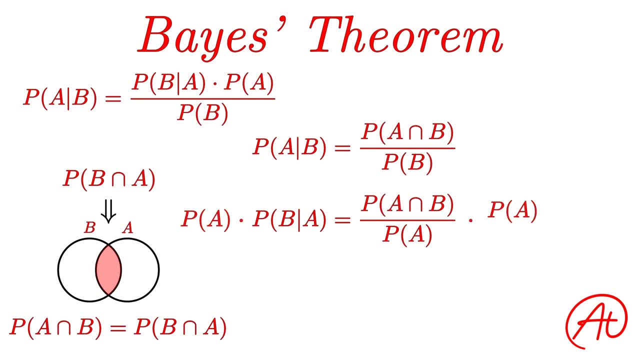 Next, we can multiply both sides of the bottom equation by the probability of A to cancel it out on the right side. This would then give us the probability of A times the probability of B, given A is equal to the probability of A and B. Or if we were to rewrite: 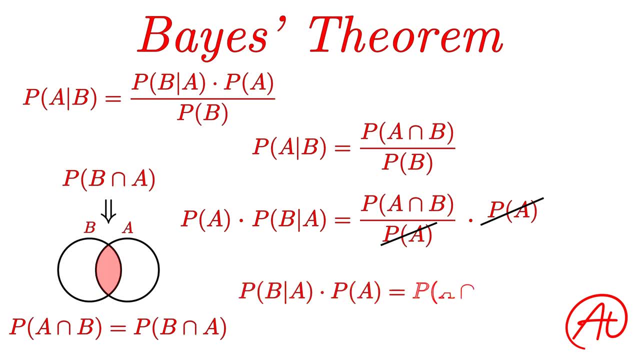 the left side. that would be the probability of B given A times the probability of A is equal to the probability of A and B. Then we can take this and substitute it into the original conditional formula to ultimately get Bayes' theorem that says the probability of A given B. 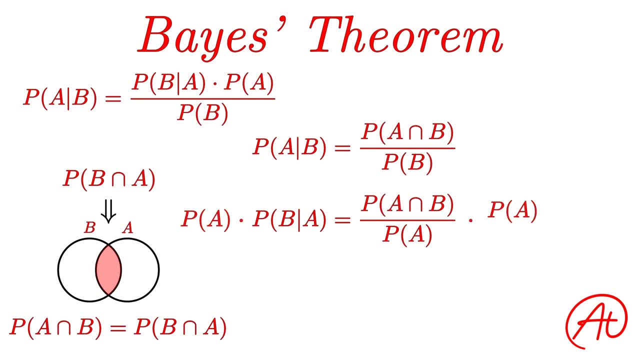 Next, we can multiply both sides of the bottom equation by the probability of A to cancel it out on the right side. This would then give us the probability of A times the probability of B, given A is equal to the probability of A and B. Or if we were to rewrite: 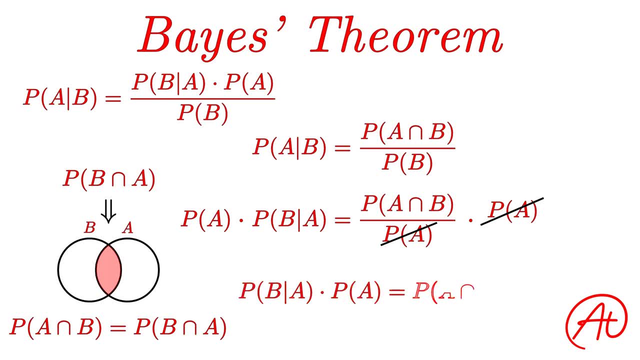 the left side. that would be the probability of B given A times the probability of A is equal to the probability of A and B. Then we can take this and substitute it into the original conditional formula to ultimately get Bay's theorem that says the probability of A given B is equal to the 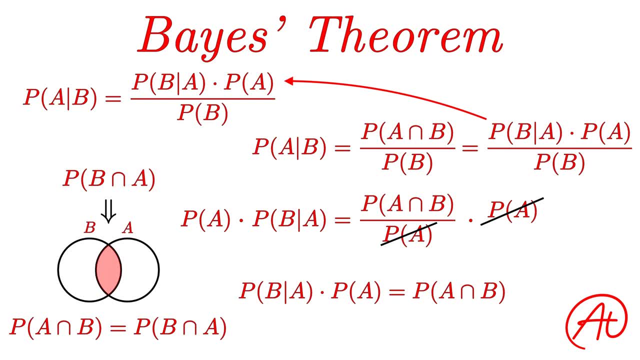 probability of B given A times the probability of A all divided by the probability of B. Whew, okay, okay. Okay, that's enough fancy algebra for now. What the heck does this actually mean, and when would we ever use this? 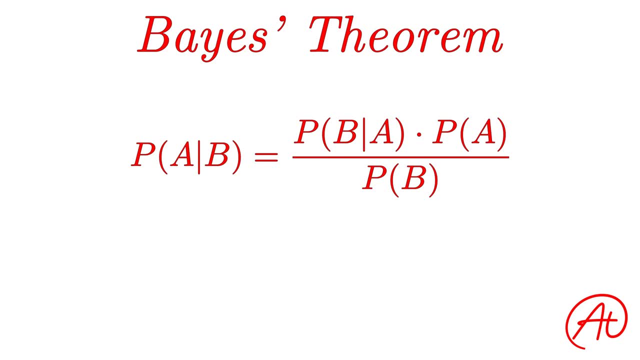 This equation is actually really useful when we want to refine our estimates for certain events occurring, when we know some additional information about the scenario. To see what I mean, let's see how we can use Bayes' theorem in an example. Let's say you've been planning a picnic for your family. 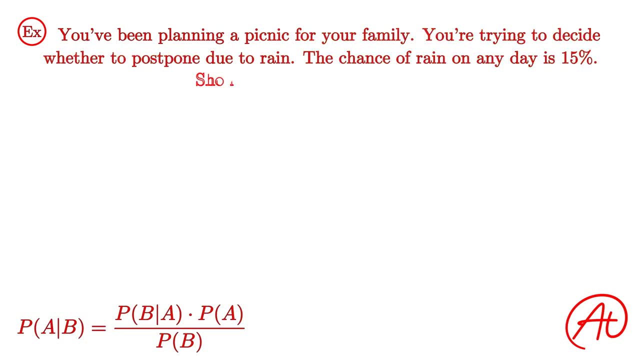 The morning of the picnic you're worried about rain and you're trying to figure out whether you should postpone or not. Let's say you know that in your area the chance of rain on any given day is 15%, or in other words the probability of rain is 0.15.. 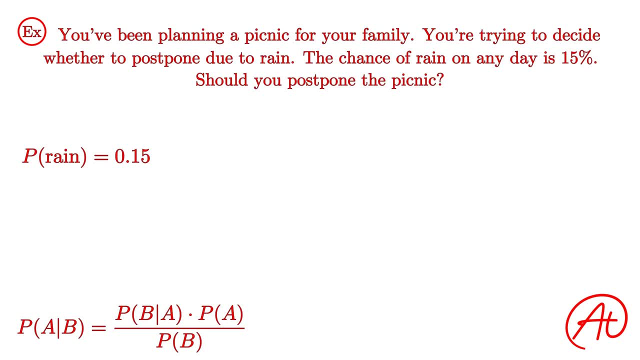 If you were to only go off this information, you might also say there's a 15% chance of it raining today, and that that's sufficiently low for you to feel confident in still having your picnic. This is a great initial guess, but is there a way we could make an even more informed? 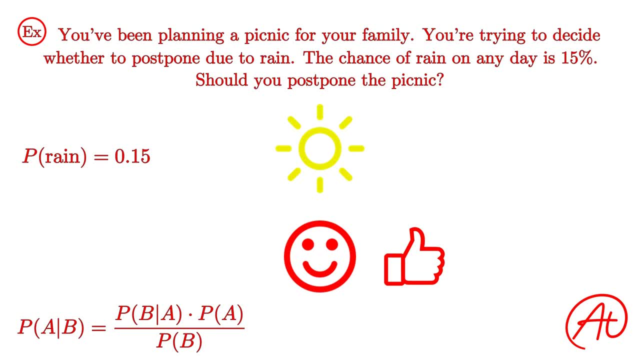 decision. Well, one thing you might do is go outside and see if it's cloudy or not. If it's a clear day, you might feel even more confident that it won't rain, Or if it's very cloudy, you might even be more worried that it'll rain. 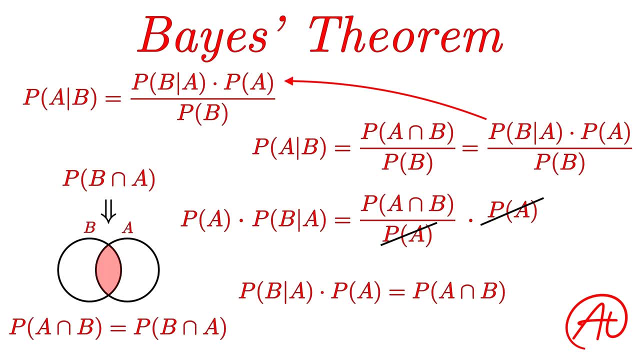 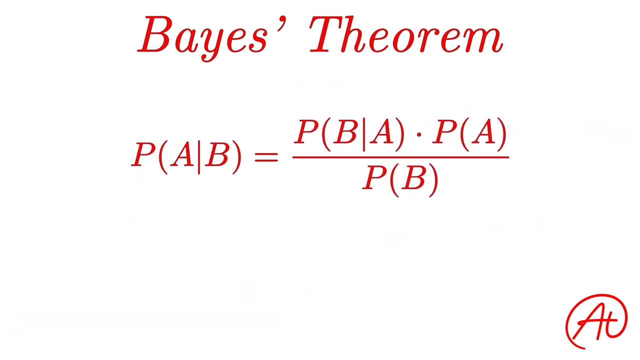 is equal to the probability of B, given A times the probability of A all divided by the probability of B. Whew, okay, That's enough fancy algebra for now. What the heck does this actually mean, and when would we ever use this? Well, this equation is actually really useful when we 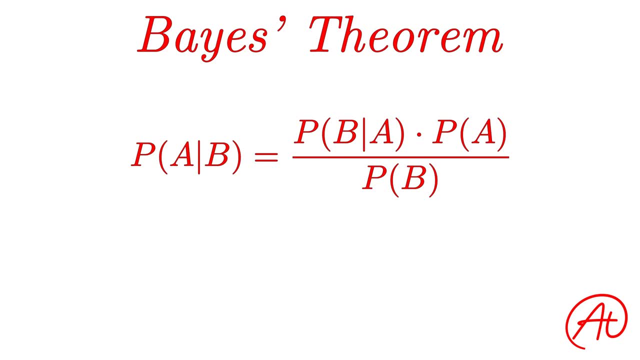 want to refine our estimates for certain events occurring when we know some additional information about the scenario. To see what I mean, let's see how we can use Bayes' theorem in an example. Let's say you've been planning a picnic for your family. 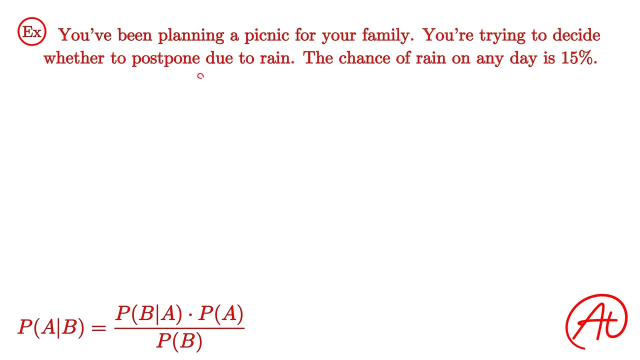 The morning of the picnic you're worried about rain and you're trying to figure out whether you should postpone or not. Let's say you know that in your area the chance of rain on any given day is 15 percent, or in other words the probability of rain is 0.15.. If you were to only go off this? 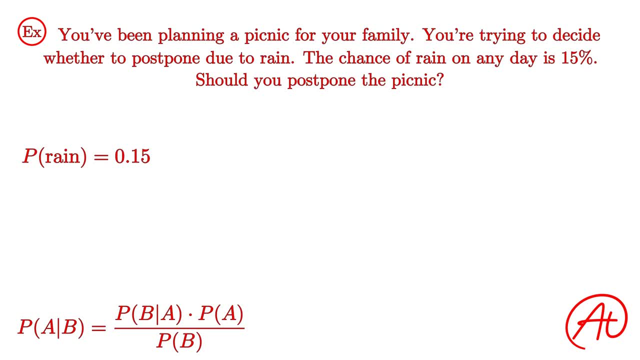 information. you might also say there's a 15 percent chance of it raining today, and that that's sufficiently low for you to feel confident in still having your picnic. This is a great initial guess, but is there a way we could make an even more informed decision? 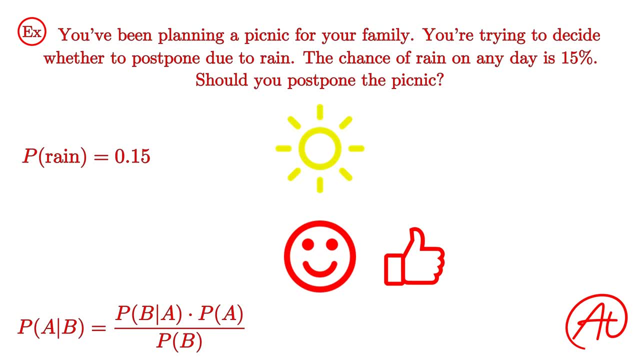 Well, one thing you might do is go outside and see if it's cloudy or not. If it's a clear day, you might feel even more confident that it won't rain, or if it's very cloudy, you might even be more worried that it'll rain. 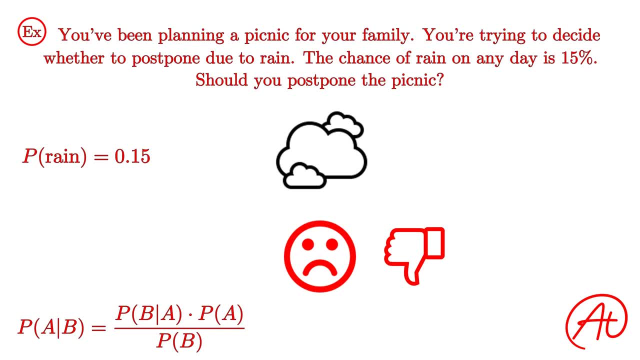 This is something that we would intuitively think to do, but this is exactly what Bayes' theorem helps with. It helps you calculate the probability of something occurring when you already have some additional information about the scenario. For this example, let's say that on the morning of 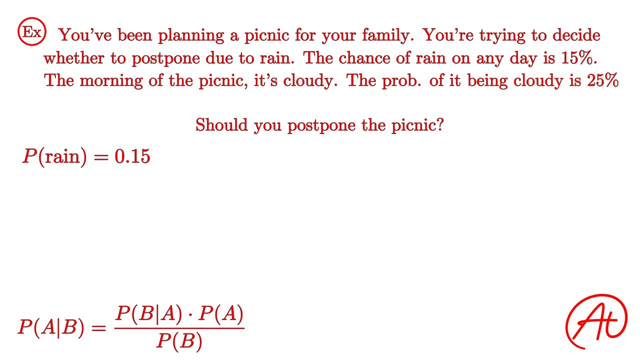 the picnic. when we were planning a picnic for our family, there was a chance of rain and we wake up. we find that it's cloudy outside. We know that the probability of it being cloudy in the morning on any given day is 25 percent or 0.25.. You also happen to know that on days when it does, 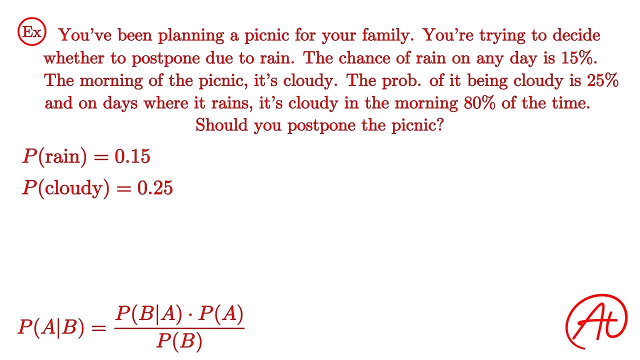 end up raining. it is cloudy in the morning 80 percent of the time, or, in other words, the probability of it being cloudy in the morning, given that we know it ends up raining, is 0.8.. Using this additional information and our newfound knowledge of Bayes' theorem, 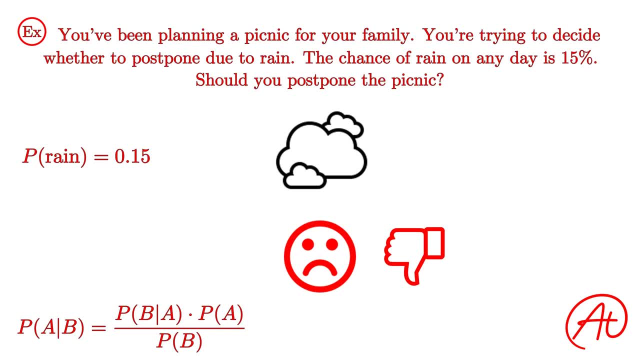 This is something that we would intuitively think to do, but this is exactly what Bayes' theorem helps with. It helps you calculate the probability of something occurring when you already have some additional information about the scenario. For this example, let's say that on the morning of the picnic, when you're planning a picnic, 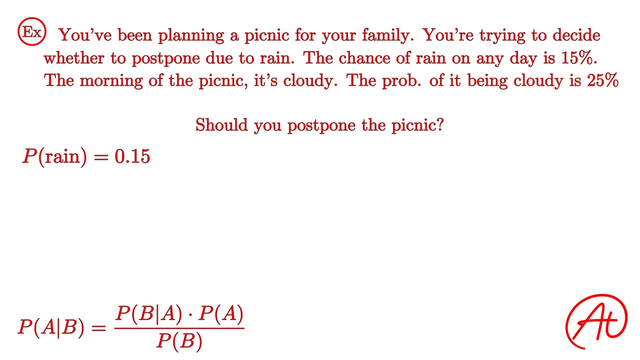 when we wake up, we find that it's cloudy outside. We know that the probability of it being cloudy in the morning on any given day is 25% or 0.25.. You also happen to know that on days when it does end up raining, it is cloudy in the. 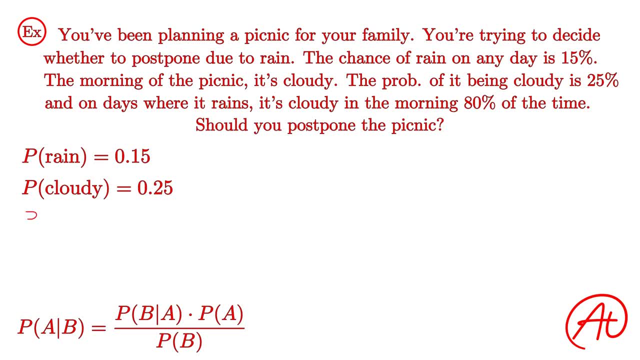 morning 80% of the time, Or, in other words, the probability of it being cloudy in the morning, given that we know it ends up raining- is 0.8.. Using this additional information and our newfound knowledge of Bayes' theorem, we'll 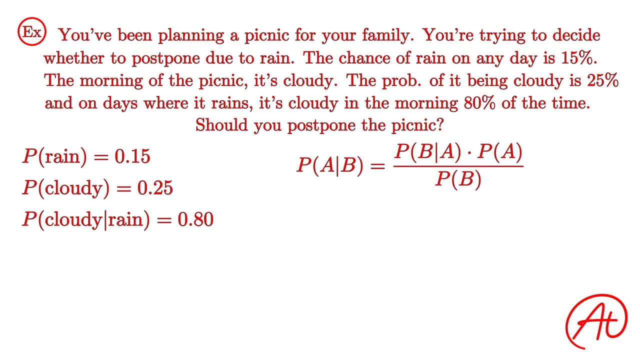 be able to calculate an even better estimate for the probability of it raining during the picnic, Rewriting the equation in terms of the events being cloudy in the morning and raining later in the day. we would then get that the probability of it raining during the picnic, given that 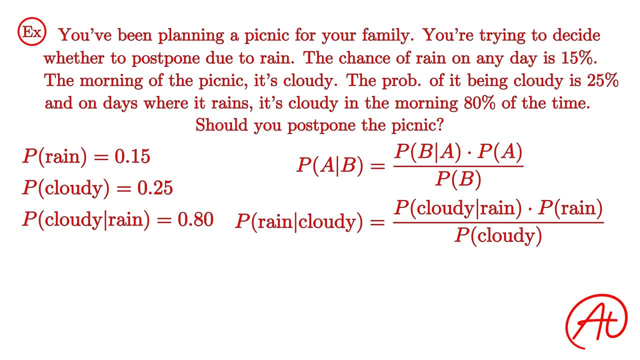 it's cloudy in the morning is equal to the probability of it being cloudy in the morning, given that it rains times the probability of it raining in general all divided by the probability of it being cloudy in general. Playing with numbers, Plugging in the values that we know, we would get that the probability of it raining during. 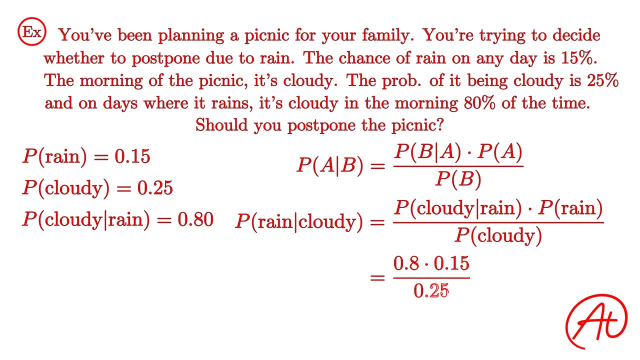 the picnic, given that it was cloudy, is equal to 0.8 times 0.15, all over 0.25.. Plugging this into our calculator, we get that the probability of it raining during the picnic, given that it's cloudy in the morning, is 0.48.. 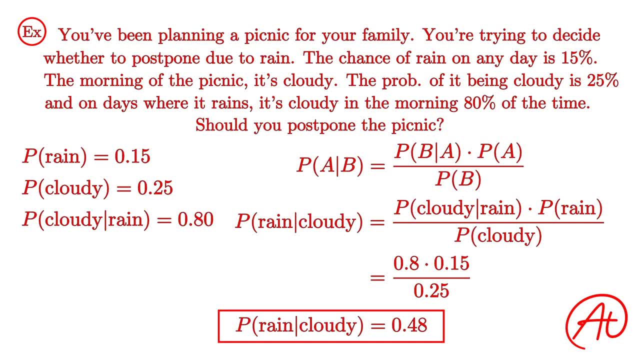 This means that the probability of it raining later during the picnic is actually over three times as likely, compared to our initial guess of 0.15, when we account for the fact that it's cloudy in the morning, With a 48% chance of it raining. given that it was cloudy, let me know down in the comments. 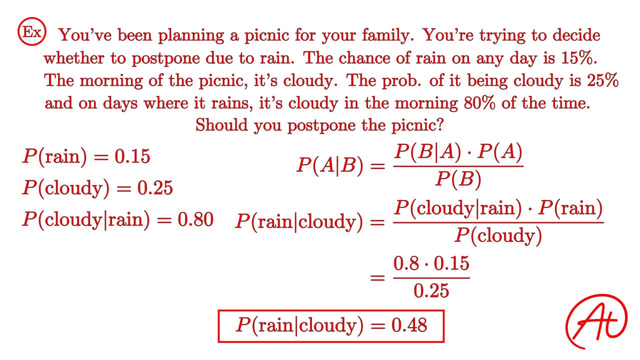 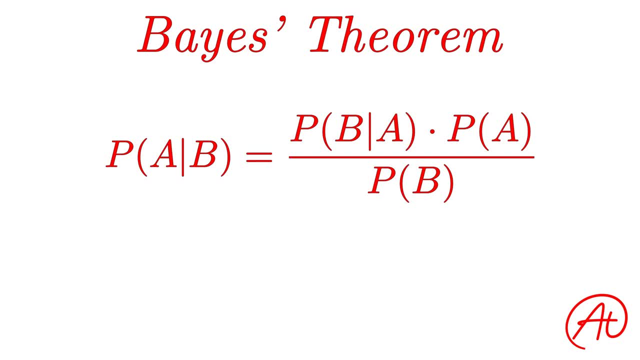 whether that would make you worried enough to reschedule your picnic or not. So that's Bayes' Theorem. I hope I was able to demystify this concept a bit and show you how and when it actually gets used in the real world. but with that being said, I know this concept can be pretty. 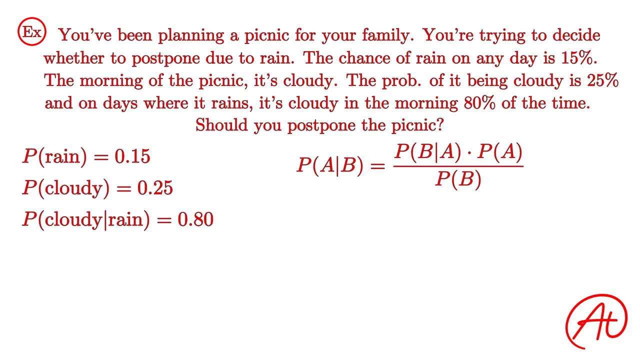 we can calculate an even better estimate for the probability of it raining during the picnic, Rewriting the equation in terms of the events being cloudy in the morning and raining later in the day. we would then get that the probability of it raining during the picnic, given that it's 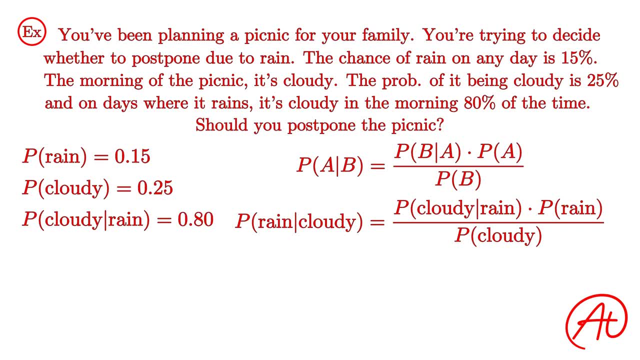 cloudy in the morning is equal to the probability of being cloudy in the morning, given that it rains times. the probability of it raining in general all divided by the probability of it being cloudy in general. Rewriting in the values that we know, we would get that the probability of it raining during the 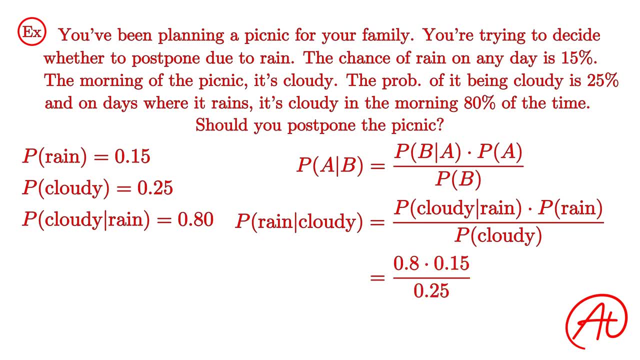 picnic, given that it was cloudy, is equal to 0.8 times 0.15, all over 0.25.. Plugging this into our calculator, we get that the probability of it raining during the picnic, given that it's cloudy in the morning, is 0.48.. This means that the probability of it raining 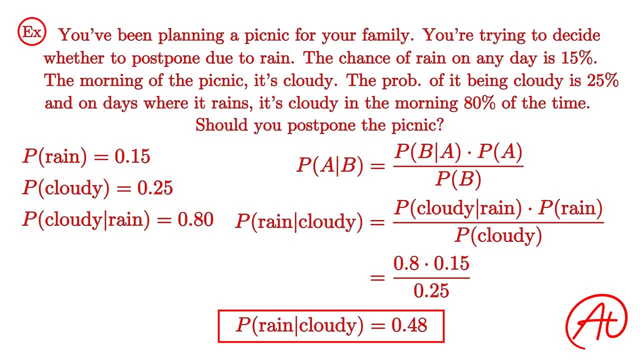 later during the picnic is actually over three times as likely compared to our initial guess of 0.15. When we account for the fact that it's cloudy in the morning, with a 48% chance of it raining. given that it was cloudy, let me know down in the comments whether that would make you. 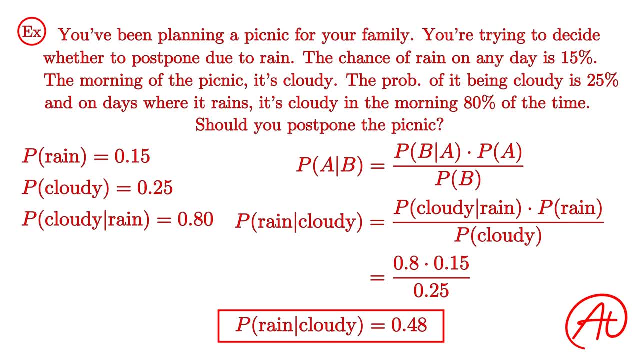 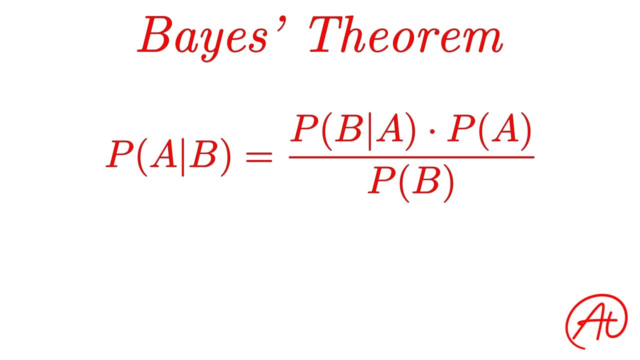 worried enough to reschedule your picnic or not. So that's Bayes' theorem. I hope I was able to demystify this concept a bit and show you how and when it actually gets used in the real world. but, with that being said, I know this concept can. 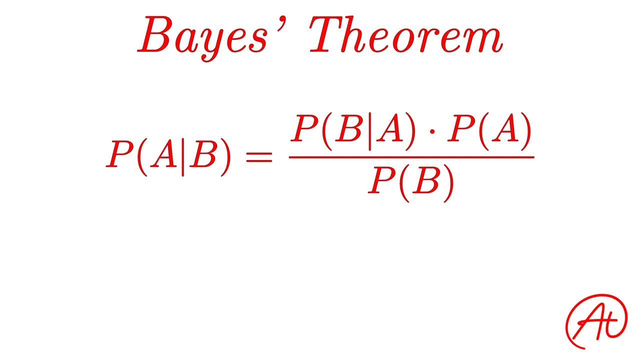 be pretty confusing, so if you're still struggling with it, I encourage you to rewind a few minutes to take a look again where this formula is. If you found this video helpful, please hit that subscribe button to support us making more videos for you. If you didn't, please leave us a comment down below to let us know what we can do better. 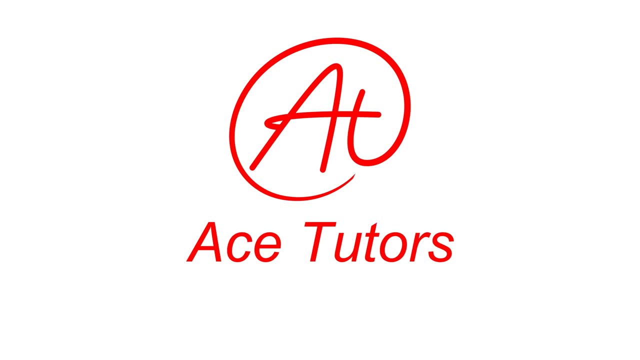 Thanks again for watching and remember you have big dreams. don't let a class get in the way you.